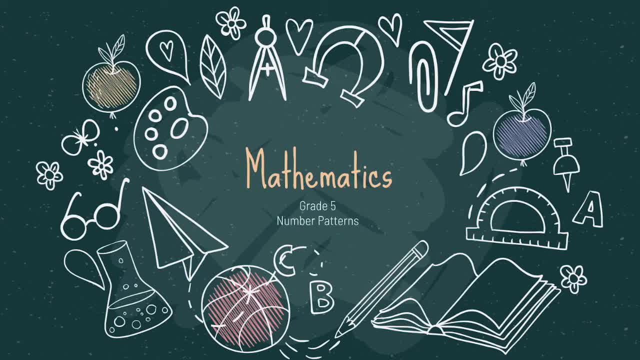 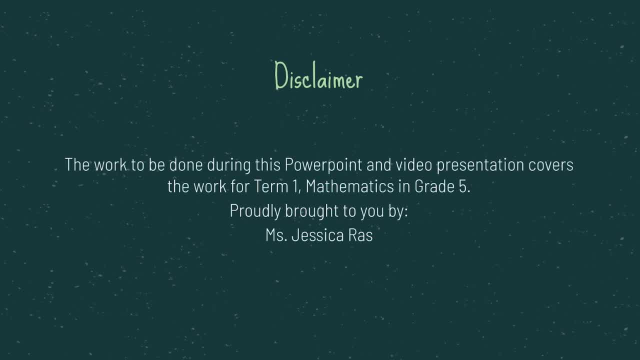 Hello Grade 5s and welcome back. Today we're going to look at number patterns. The disclaimer, the work to be done during this PowerPoint and video presentation covers the work for Term 1 Mathematics in Grade 5, proudly brought to you by Ms Jessica Ross. 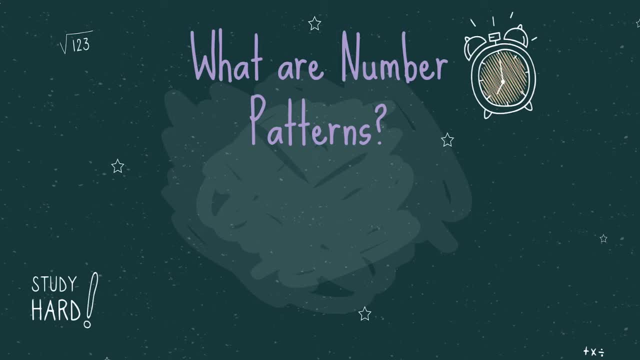 We firstly need to look at what is number patterns. Number pattern is a pattern or sequence in a series of numbers. This pattern generally establishes a common relationship between all numbers. In order to solve the problem on the number pattern first we have to understand the rule being followed in the pattern. 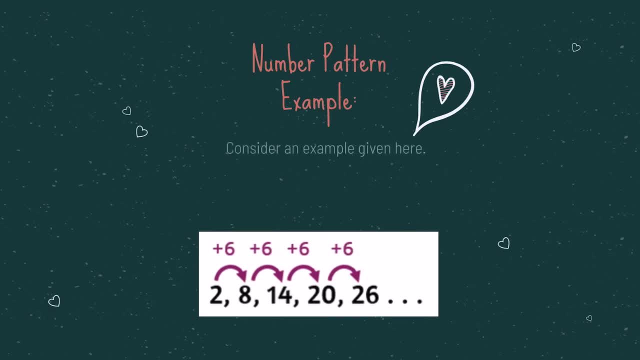 Let's look at this example. The giving sequence of numbers is 2,, 8,, 14,, 20 and 20.. So to get from the 2 until the 8, we added 6.. To get from the 8 to 14, we added 6 again. 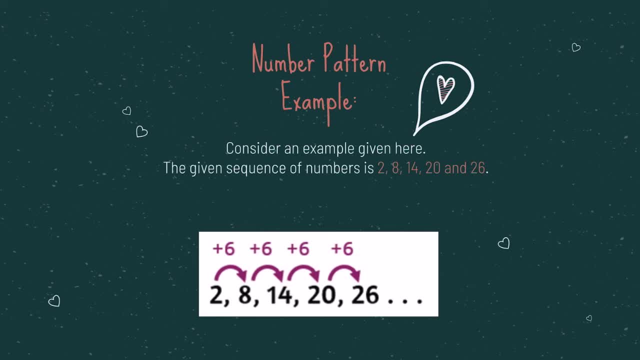 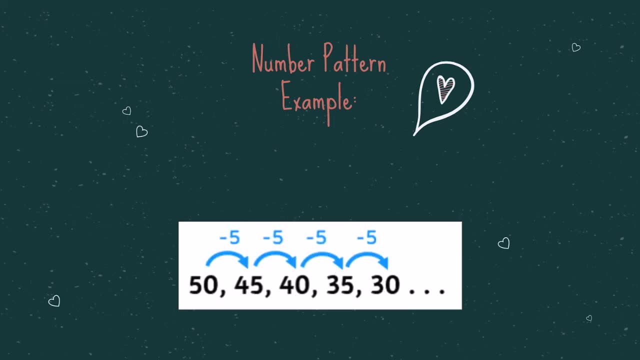 To get from the 14 to the 20, we added 6 again. So the rule is to add 6.. The next example: We have 50,, 45,, 40,, 35, and 30. So from 50 until 45, we subtracted 5.. 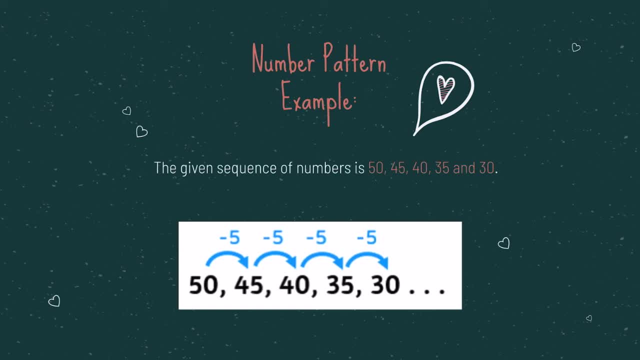 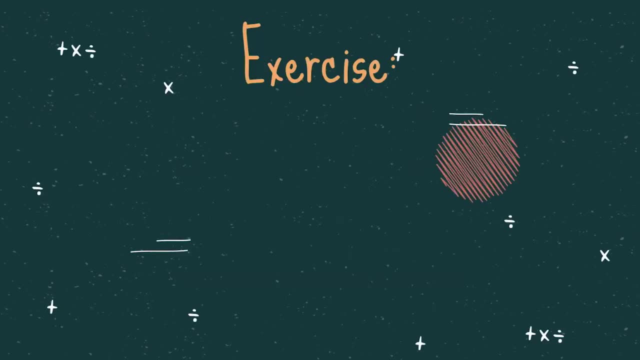 From 45 until 40, we subtracted 5 again, So the rule is to subtract 5.. The exercise that you guys will be doing today is Unit 3, Number Patterns- The Getting Started Exercise On page 21.. Please do not forget to subscribe to our channel. 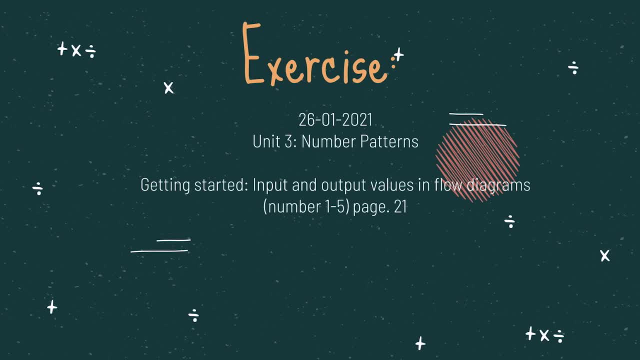 Number 1 until 5.. Remember to write the heading and the date for me. If you are done with the getting started, please draw a line underneath your work and write the heading and the date again- Activity 1 on page 22.. 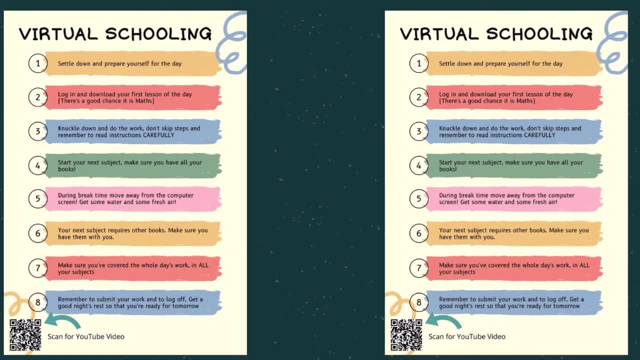 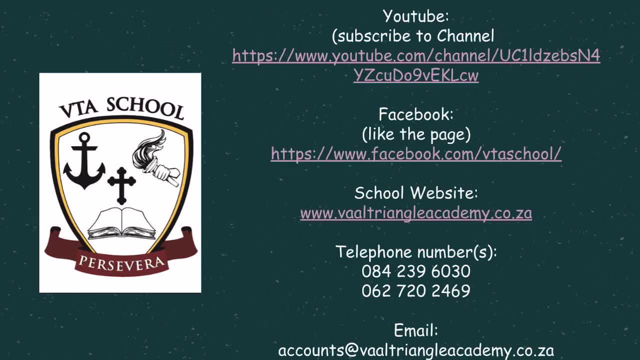 Number 1 until number 3.. This is the virtual schooling rules. Please go through it. Number 1 until 3.. Remember to write everything in your book status on the slides.